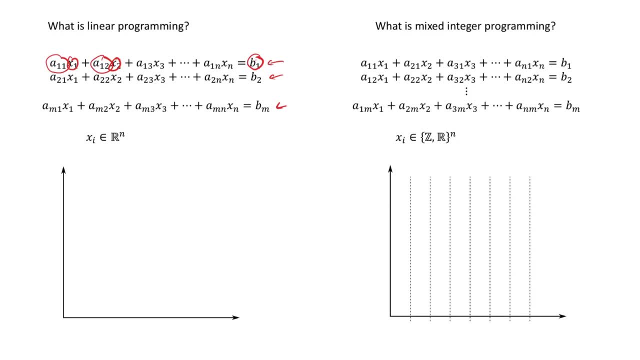 We note that these variables are in the real space or are continuous, And we do that by saying every variable x with subscript i, so that x1, i i equals 1, x2, i equals 2, and so on. 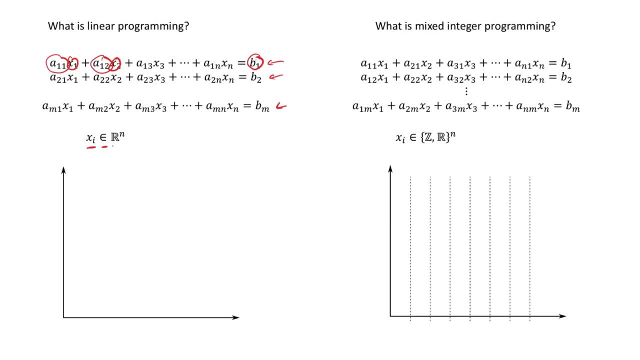 Each of those variables are in right in the space that's real of dimension n. All right, we have n variables here, So let's look at an example of two different variables and just look at what a linear program might look like. 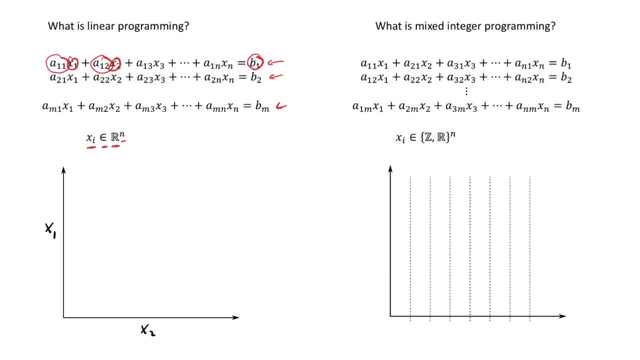 Let's say we have x1 here and x2. And we have again: it's a linear program, so you have linear equations. So we might draw our first linear equation here And this linear equation would be described by the first. let's say a11, x1 plus a12, x2 equals b2.. 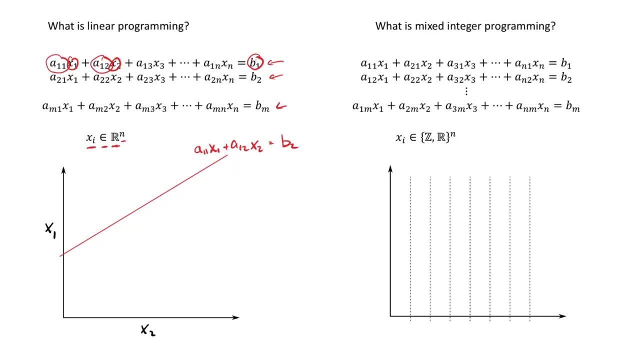 That's our first equation. And then we have, let's say, a second equation over here, And this one will be a21.. So we have a21, x1 plus a22, x2 is equal to b2.. Sorry, I miswrote this. 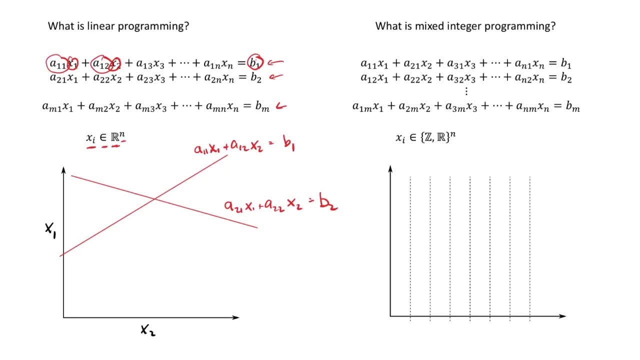 It should be b1 up here, right? So we have two equations And in this case we have two unknowns. So we can solve this equation pretty easily. And we solve it by finding the values of x1 and x2 that satisfy both equations. 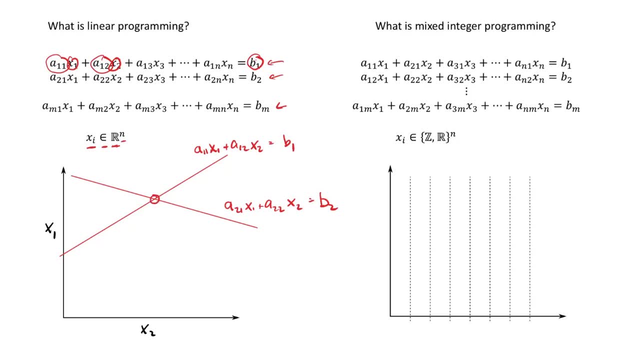 And that in this case is this point of intersection here. All right. so a linear program is a set. It's a set of equations that can be solved for one or more solutions. Now, when we talk about an integer program, 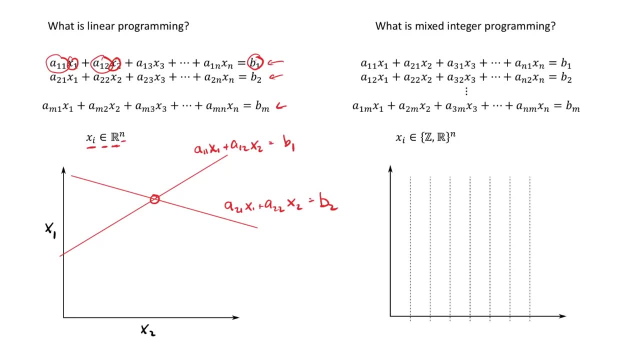 the only difference between a linear program and a mixed integer or a mixed integer linear program is that some of the variables for the integer program are integers, that they're discrete variables. So here again we have a set of equations right 1, 2 through m. 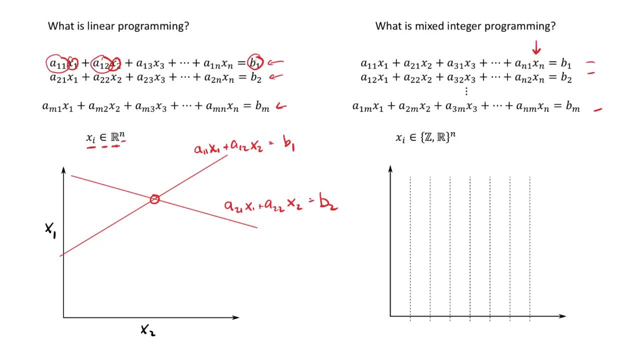 But some of these variables, let's say xn, are actually a variable that can only take on discrete values or, in this case, integral values. So an example here would be again, if we could look at plotting this out, maybe we have x1 and x2.. 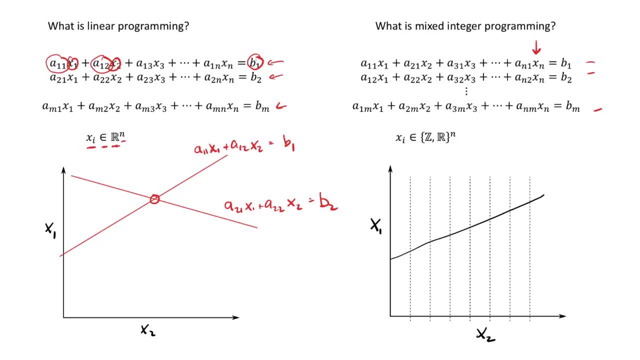 And we can draw lines again, like we had before for our constraints or for our equations, And we will then try to solve this equation for where x1 and x2 satisfy both. So what we would do is actually normally if it was an entirely linear, continuous problem. 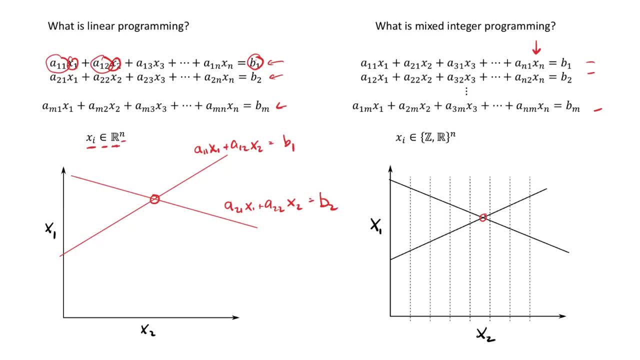 we would find the solution to be right here, where it's intersecting. However, in this case, x2 has to be an integer value, So the integers I've drawn correspond to the dotted lines. So actually, the only feasible solutions would be along the intersection of the dotted line. 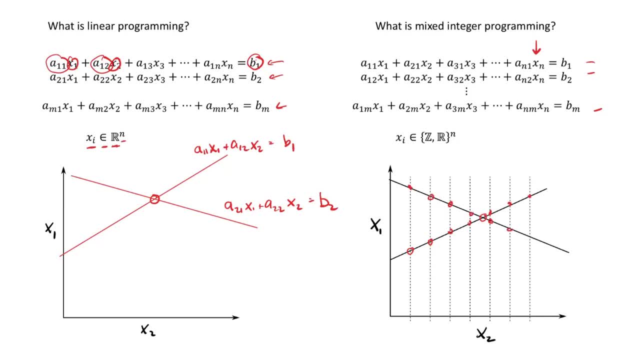 where this other line has been drawn. So, if you look at this, actually there's no solution here because there's no single set of x1 and x2 that actually satisfy the constraints or the equations that we've written out. So we'll talk a little bit about how to deal with this, how to deal with integer programs. 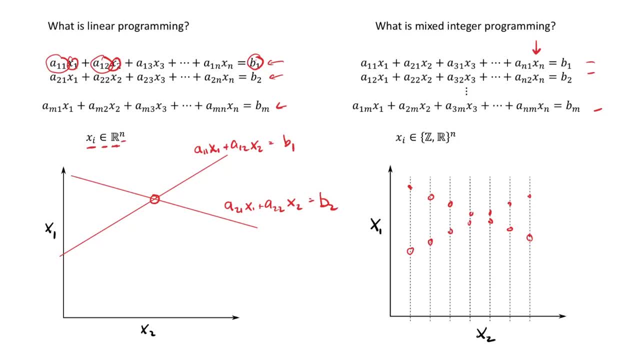 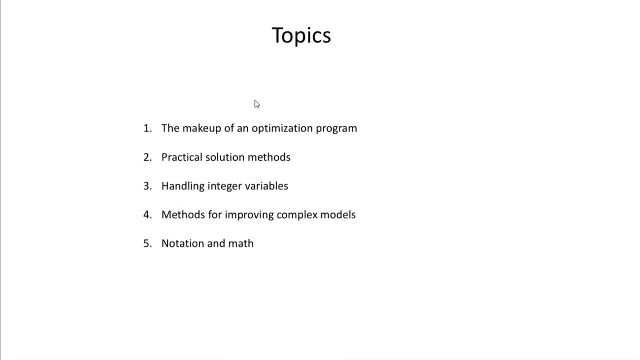 The reason why you're going to want to use integers is because they allow you to compare different, distinct modes of operation or procedures that you might run into A quick overview of the topics we're going to go through in this set of videos. First we'll go over the makeup of the optimization problem: optimization program. 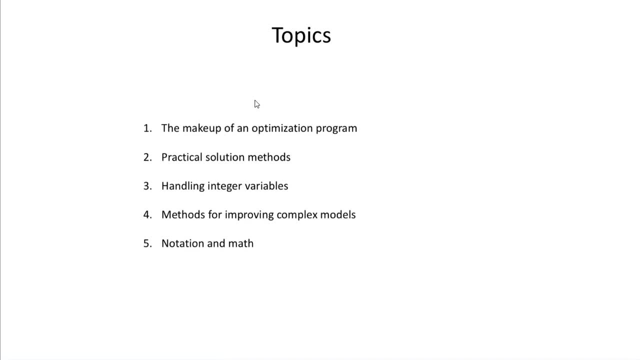 what are the pieces that we need to talk about? Second, we'll go through practical solution methods. Third, we'll go through how to handle integer variables. We'll start with simpler examples where everything is continuous and then go to integer variables. 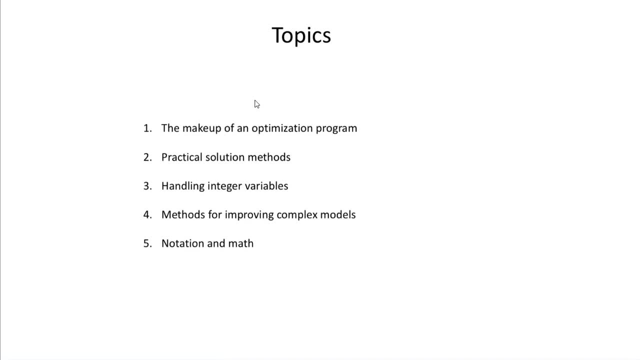 Then we'll talk about methods for improving complex models. Naturally, the reason why you might want to use these models is because they scale very well. You can write a set of equations in a compact way and scale them up so that they're automatically handling thousands of constraints and variables at the same time. 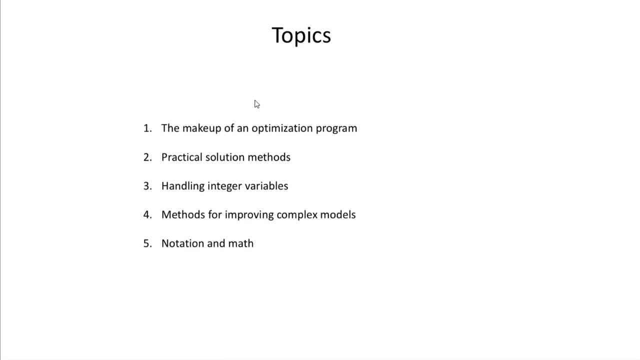 But when you do that, you're going to have a lot of problems. To do that, you need to keep several things in mind, and we'll talk about what those are. Finally, I'll give you just a quick overview of common notation and math that's used to write out these problems. 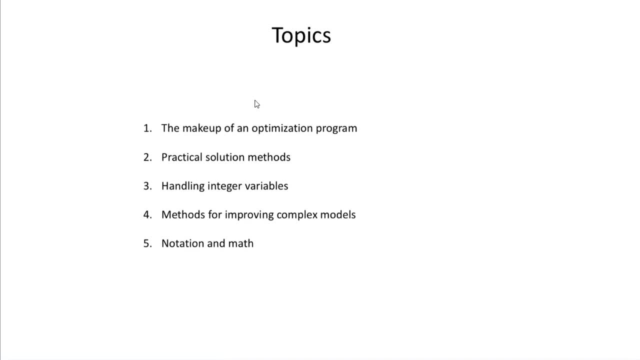 It becomes more and more important, as the problems grow, to be careful about how you're, say, writing indices or representing sets or variables or things like that. So we'll just quickly go over what's needed in order to express your linear integer program, in case you have any questions. 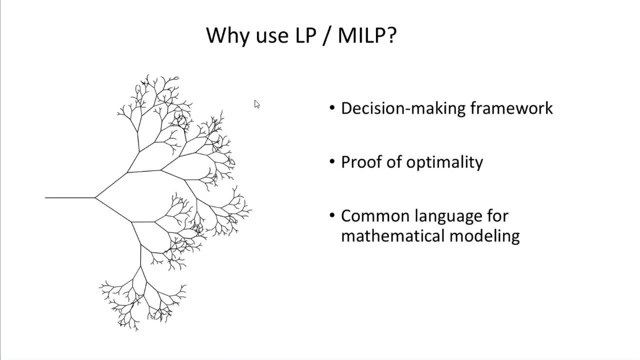 So let's talk a little bit about why you'd want to use linear programming or mixed integer programming. So let's imagine that you're in a scenario where you have a complicated decision to make. Let's say you're trying to come up with a schedule of production from some system. 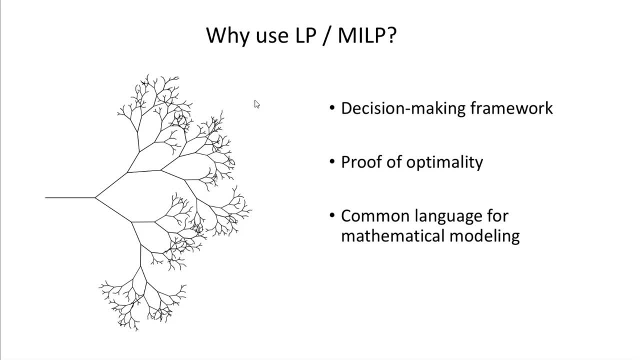 Maybe you run a plant that makes some widget and you want to produce that widget according to some schedule. But you have to think about when you're going to use it, When the parts that make the widget are coming in, when your labor is available. 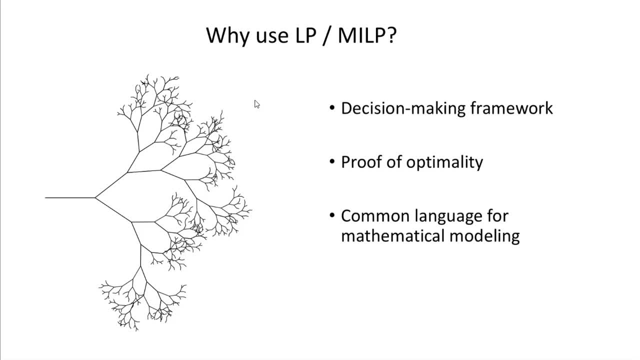 what you expect to be able to sell, as a function of time, et cetera. So you have this complicated decision that varies in time, and so you might, as a human, start off by going along this decision tree and deciding: okay, well, first thing I'm going to do is make parts tomorrow. 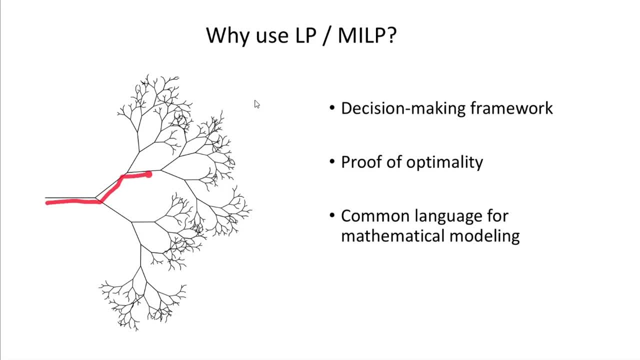 And then second thing I'm going to do is order new pieces on Thursday and so on, And you just keep going down this tree and eventually you come to some decision where you believe you've done a pretty good job, just based on the information you had on hand as you were going through the process. 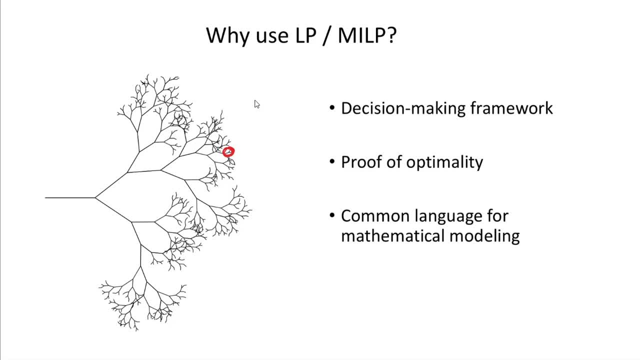 But you really don't know whether or not that answer that you came up with is the optimal one, or even that close. You used rules of thumb, or what we call heuristics, in order to make judgments about which way to go at each branch along the way. 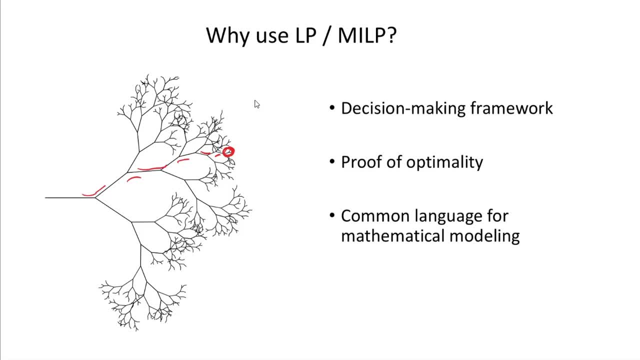 And, ultimately, you ended up with a decision. What linear programming or mixed integer programming does for you is: it provides a rigorous, systematic way of searching all the possible outcomes, or traversing through the tree, in other words, in order to get you to an outcome that is optimal. 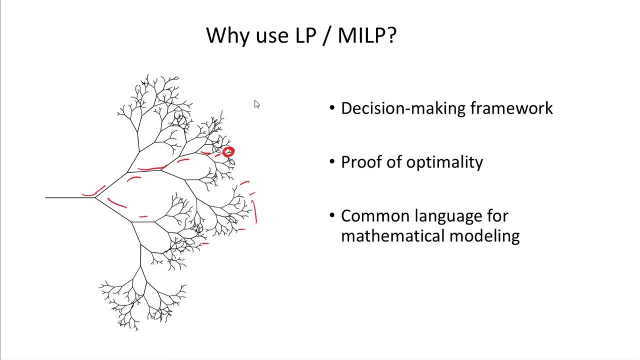 One of the battles, though, is when you come to the end of the tree. you've made all the decisions there are to make. How do you even know whether that is an optimal solution or not? Linear programming and mixed integer programming have built in. 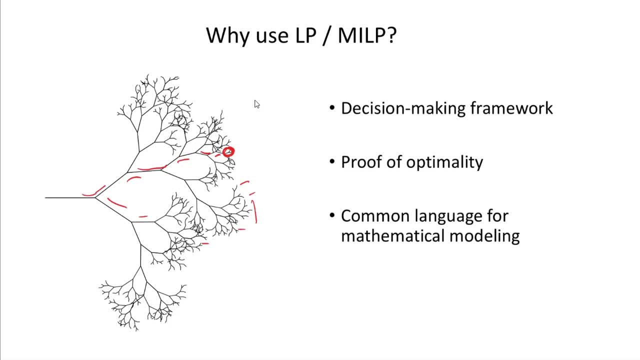 Methods that give you proof of optimality, So you at the end of the tree will know whether or not the answer you have is an optimal one. The last thing, the last reason why you might want to use LP or MLP, is that it's really useful to have a common language for mathematical modeling. 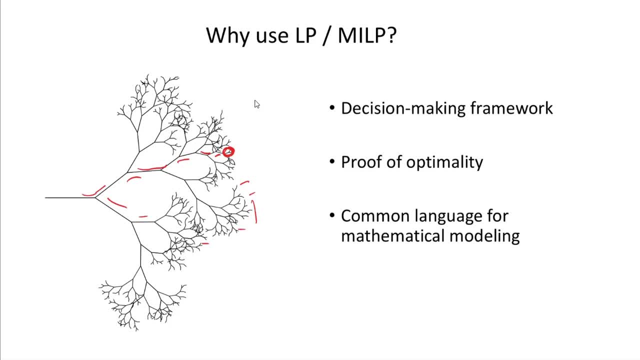 So when we're talking about solving large sets of equations, and particularly sets of equations where we're trying to optimize some objective, we generally, generally need a common language so that we can communicate our results, make use of advances that others have made, and so on. 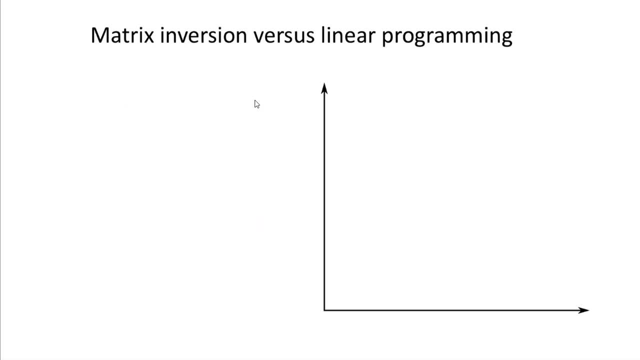 So these techniques provide that. The last thing you might be wondering, the last thing we'll talk about in this video is: okay, I took linear algebra. I know how to solve systems of equations. you know, I have techniques for inverting matrices or for using Gauss elimination or whatever. 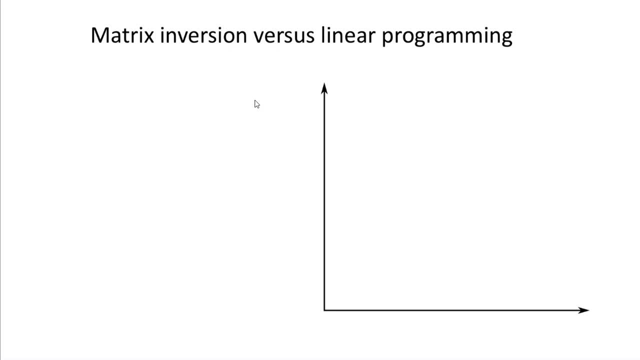 So why am I bothering with LP or MLP? Well, let's look a little bit more carefully at what linear algebra gives you when you're using the techniques that you're probably most familiar with. So let's start off and let's say we have some system of equations and 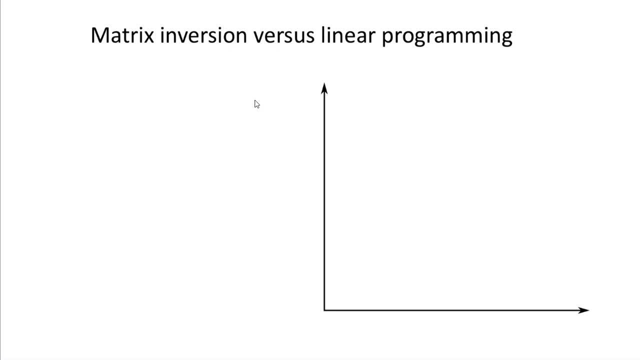 they could. you know, we could pick a three variable system of equations, which I will write out. It will be so: a 1 1, that's our constant, x 1,. a 1 2, x 2,. 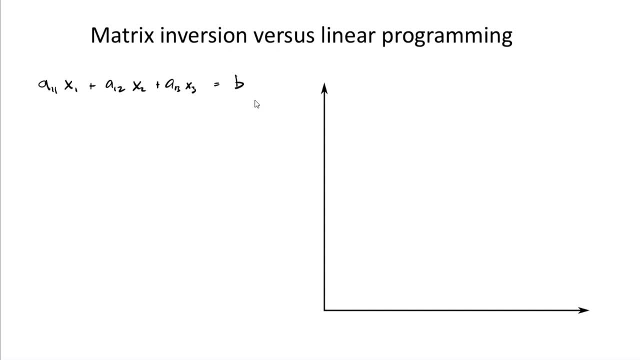 a 1, 3, x 3 is equal to b 1, right? That's our first equation. We can write the same thing for the second and third equations, which, which I'll do now. So now we have a system of three equations and three unknowns. We have right. 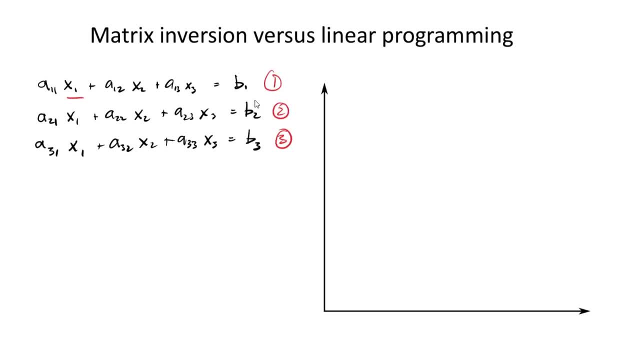 1, 2, 3 equations: 1, 2, 3, unknowns. so this has a single exact solution which we can find for x1, x2 and x3. again, you might be thinking i'll just go and use my matrix inversion, something like this, where you say: 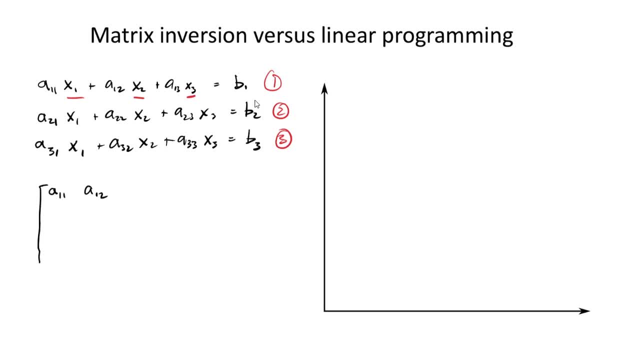 my first equation is a11, a12, a13, my second is a21, and so on. right, you fill in this matrix with your, with your constants, and then we're multiplying that by some x vector, x1, x2, x3, and then on the right hand side, we have our b vector, b1, b2, b3, and i can solve this by saying: all right, my x vector. 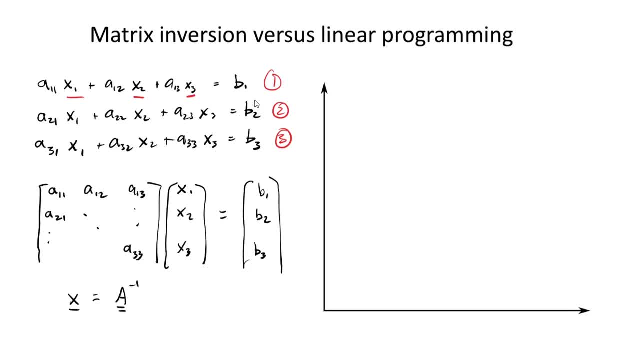 is going to be the inverse of my a matrix, my square a matrix times b, and that will give me an exact solution for x. however, what this doesn't do is deal with situations where you have more equations than you have unknowns, and that's really the key to linear programming. so here's an example. let's 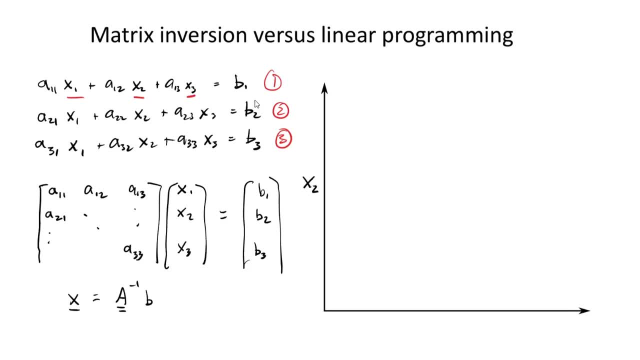 say i take this to two dimensions. right again i have x2 and x1 and i can draw my my lines again where i have a solution that i'm trying to get. so this is kind of what we had before, where our solution was x1 and x2 and x3 and x4 and x5 and x6 and x7 and x8 and x9 and x10 and x11 and x12 and x12 and 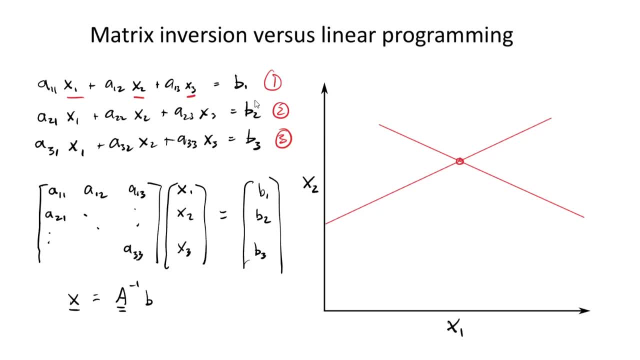 x13 and x12 and x13 and x14 and x15 and x16 and x20 and x19 are actually going to have one solution that's going to be similar to the one that you had earlier. that you had earlier, so the solution would be at the intersection of these two points. so what happens if you have a constraint that you 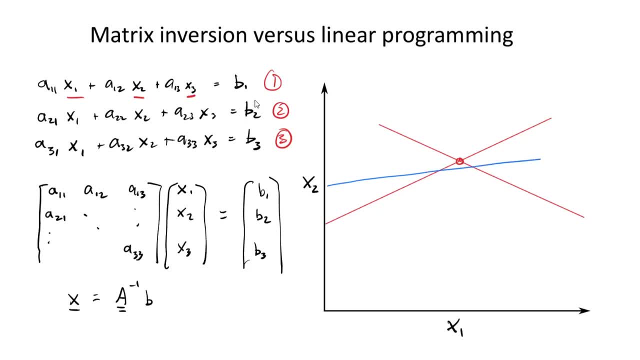 add to this problem, or another equation that you add to this problem. that's like this: right, so now i actually have, instead of one solution, i have one, two possible solutions. right, this solution and this solution. now, this as i've written, it does not quite make sense, because we have a fine integral of 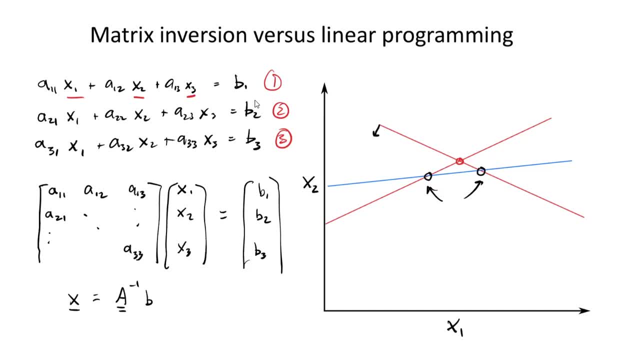 this solution and this solution, right. so i have one or two possible solutions. all right, that's one to introduce inequality, right. we have to say, all right, this is, uh, the solution has to be less than or equal to these lines. right, so we're anywhere. less than or equal to those lines is a feasible. 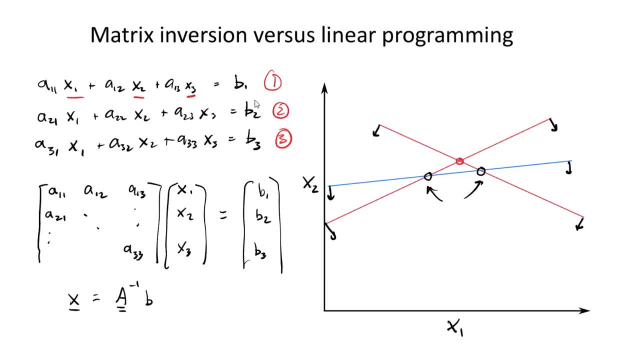 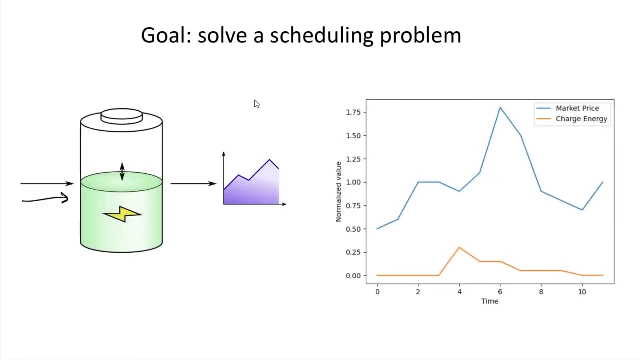 solution um, but nonetheless, you have this system of three equations with two variables and you end up with multiple solutions. so what linear programming will do is it will give you tools to systematically compare this solution here with this solution here or any other possible solutions that you might have. ultimately, what we're going to do is come up with a little bit.